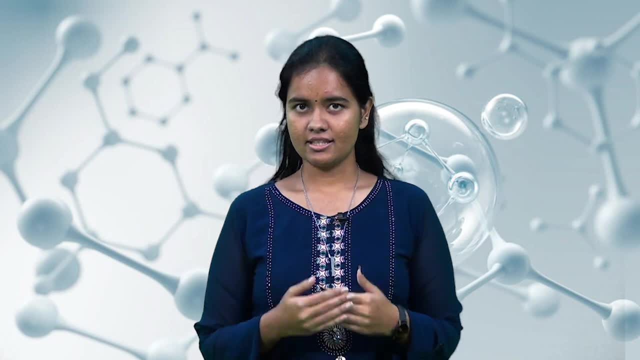 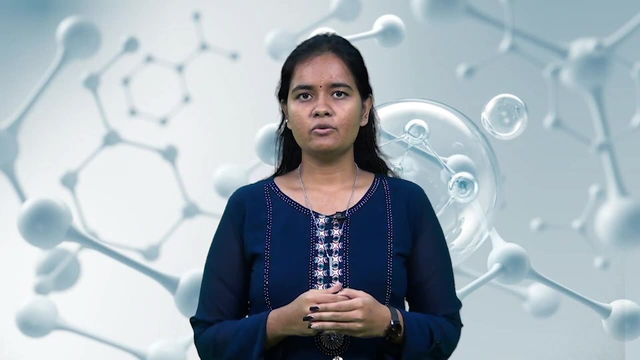 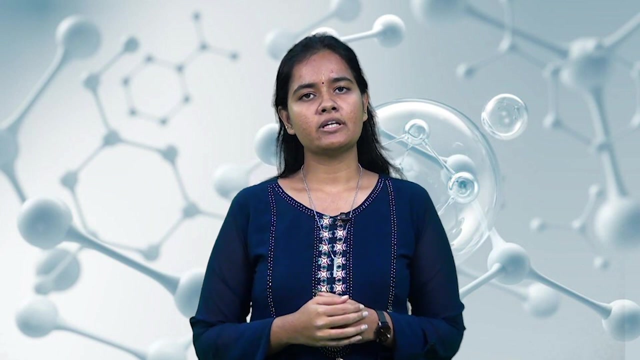 we get the result in what is called a bell curve. Now, in this experiment, we are going to take 100 readings of the radiations emitted by a radioactive source and we are going to study the nuclear counting statistics when the counts are high. We will also verify whether or not the result that we obtain at the end is a Gaussian curve or not. 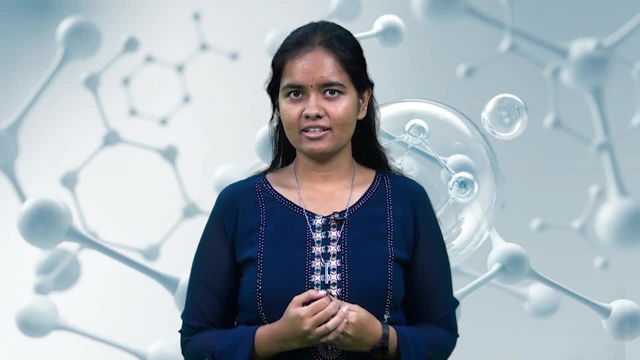 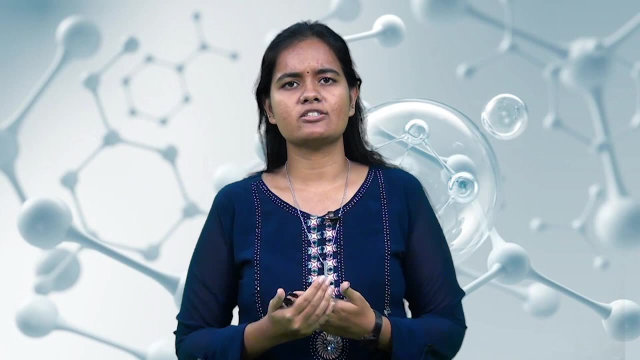 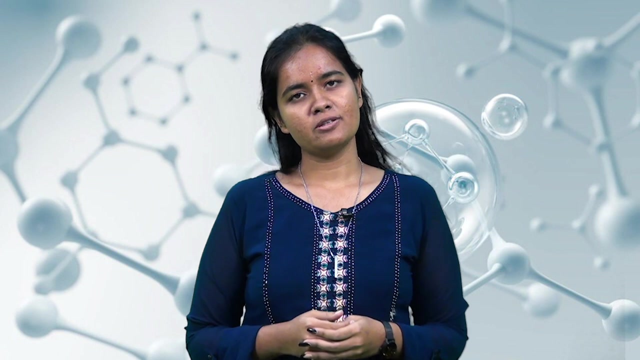 But how exactly do we count the number of radiations, of a radioactive source? So, if you remember, in the beginning of the video we were talking about GM counting systems and GM stands and GM detectors. So these GM counting systems, or Giger-Muller counting systems to be precise, is what solves our purpose. 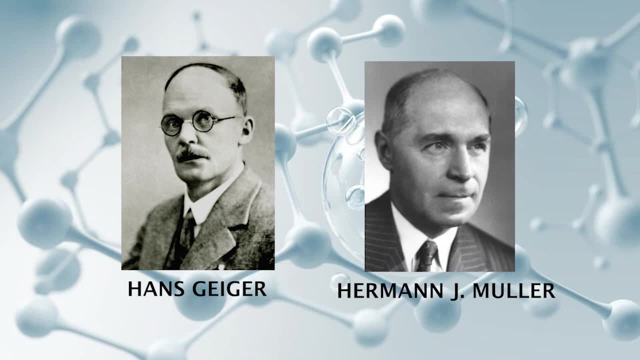 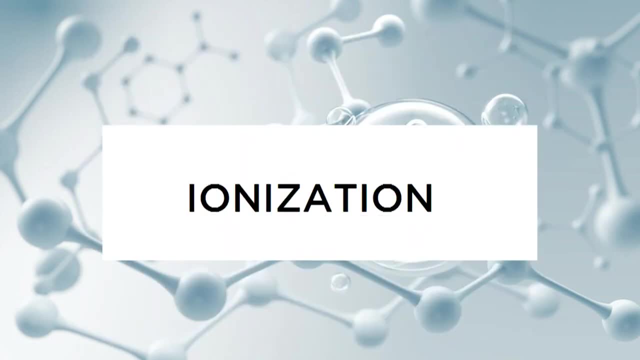 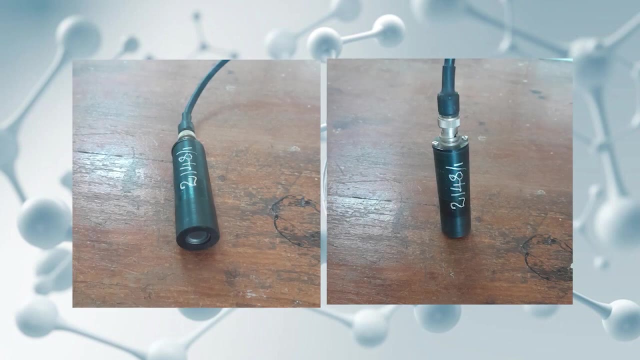 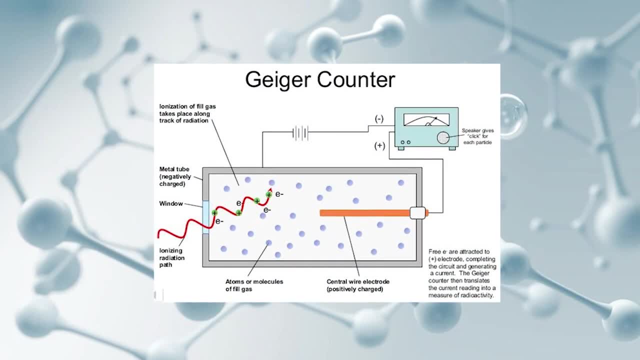 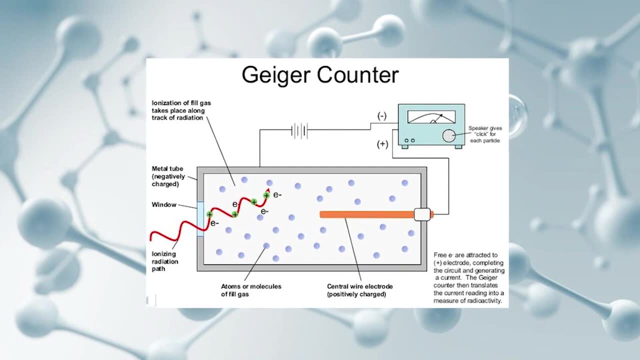 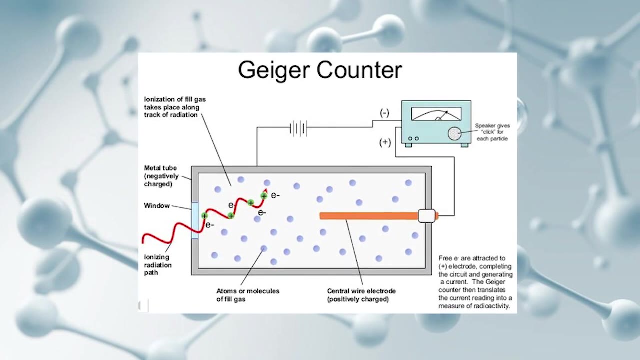 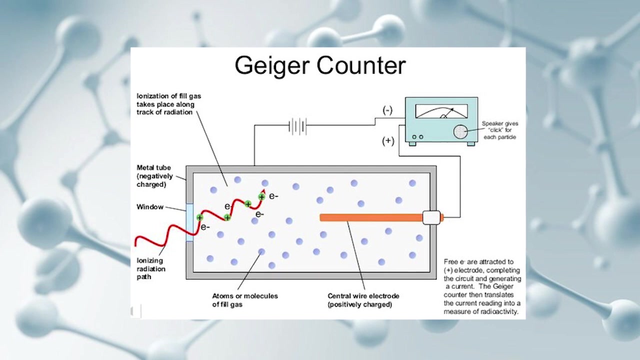 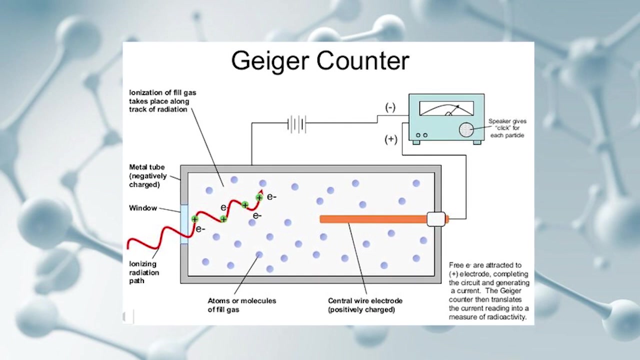 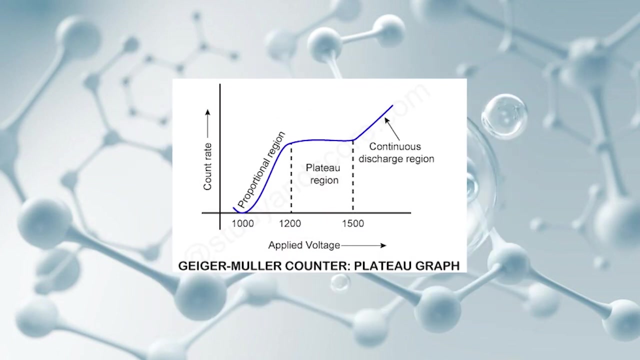 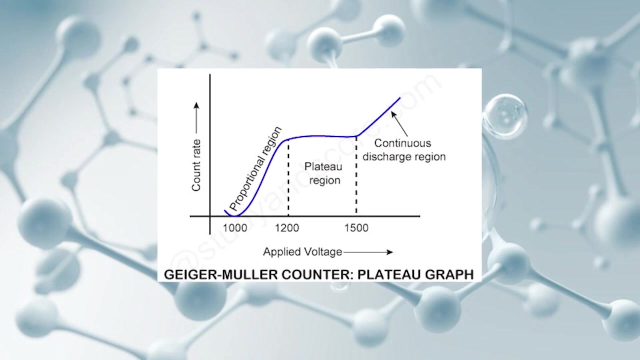 This is the cathode. This is the cathode of particles responsible for this voltage can be counted. This is how the GM counter works. There is a threshold below which the tube does not work. After this, the number of pulses is proportional to the voltage. This region is known as the proportional region. If the applied voltage 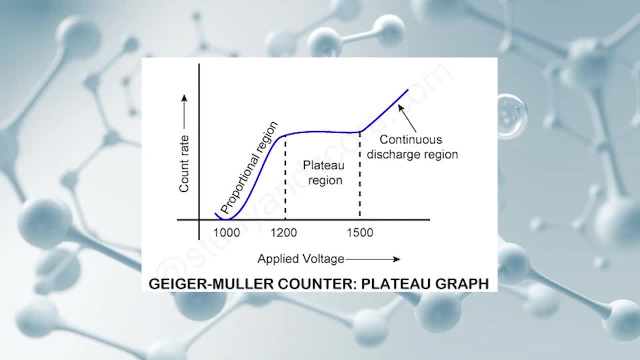 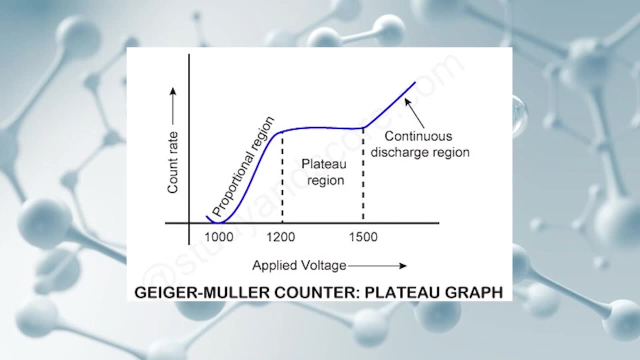 is increased further, then a point will be reached after which the count rate remains constant over a certain region. This region is known as the plateu region. This region is used for Giger-Muller Operation Beyond the plateu region, the applied 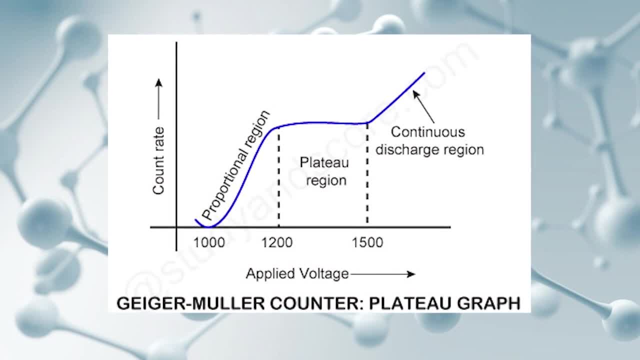 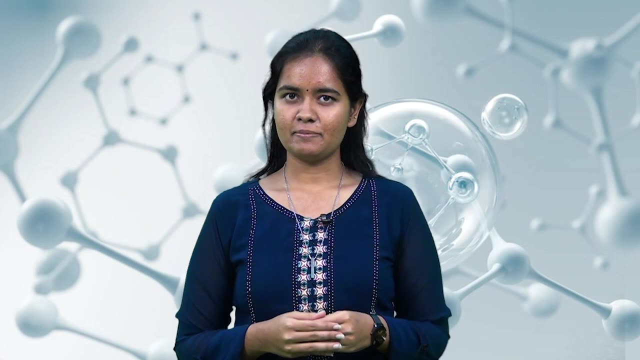 electric field is so high that a continuous discharge takes place in the tube and the count rate increases really rapidly. It does not require any ionization event to happen. So the tube must not be used in this region. That concludes the theory and principle for this experiment. 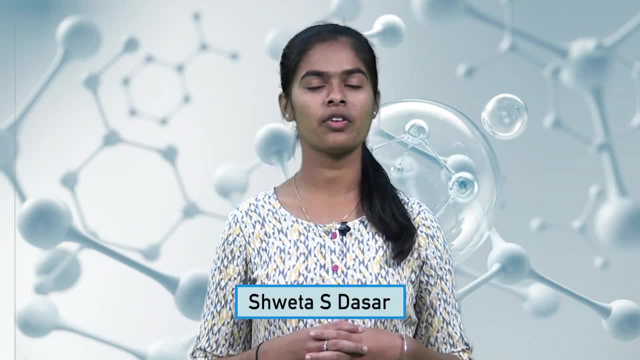 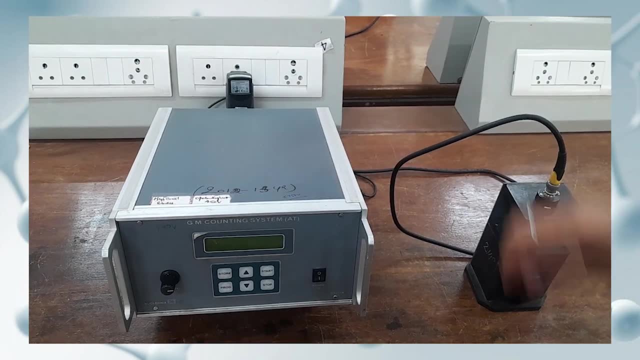 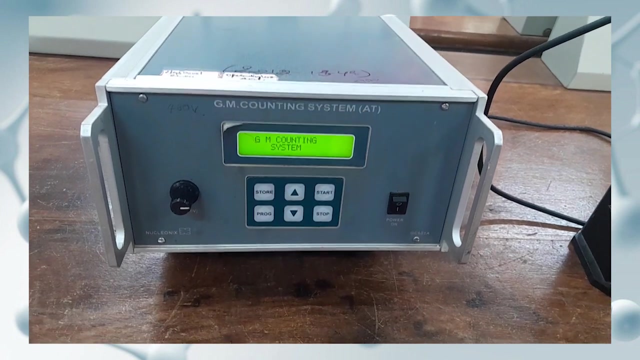 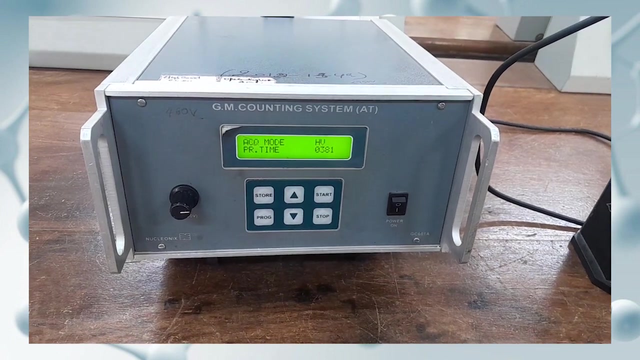 Canal iana Beta Pianine. Let us see the procedure of the experiment. First set up the GM counter in its standard procedure. Now switch on the GM counter and the power on, Then press the program button On the screen you will be able to see time and voltage. 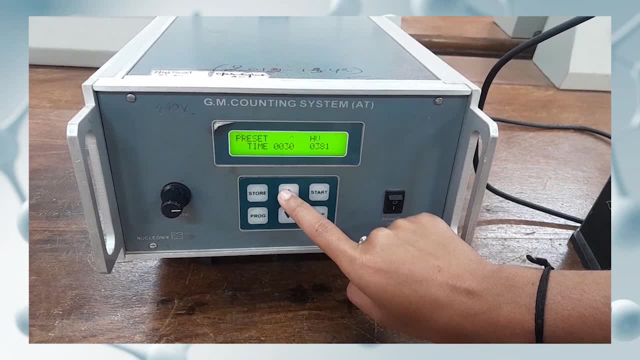 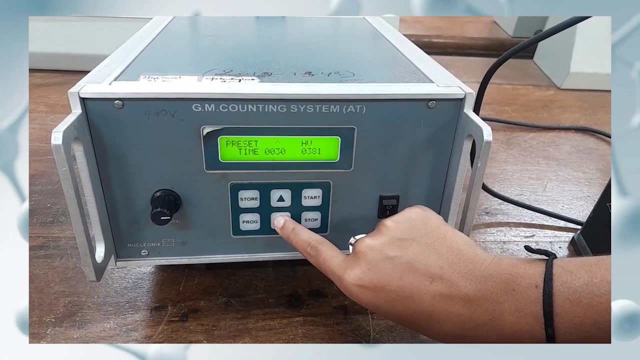 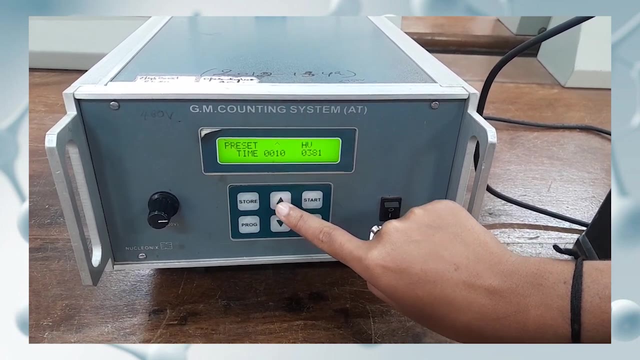 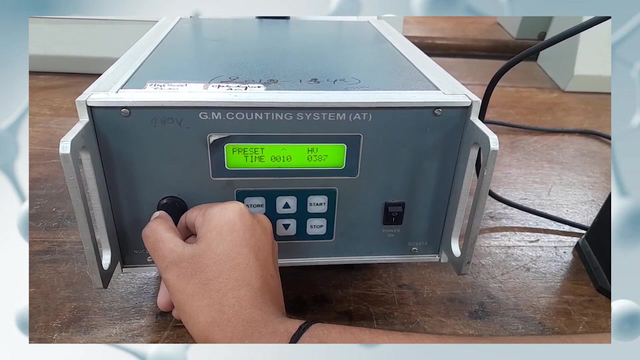 Now you have to set the time up to 10 seconds by using the arrow present on the GM counter. And now you have to set voltage up to 450 volts by using the knob given, and also ensure that you should not turn the knob very quickly. 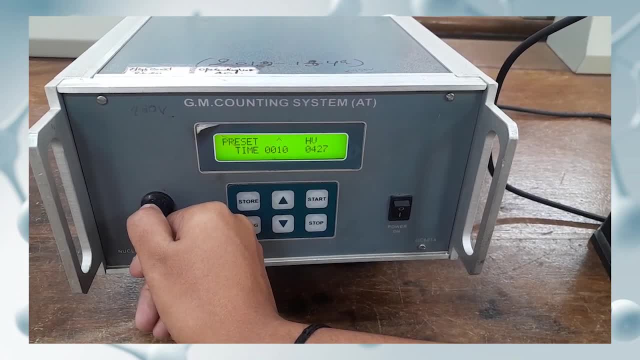 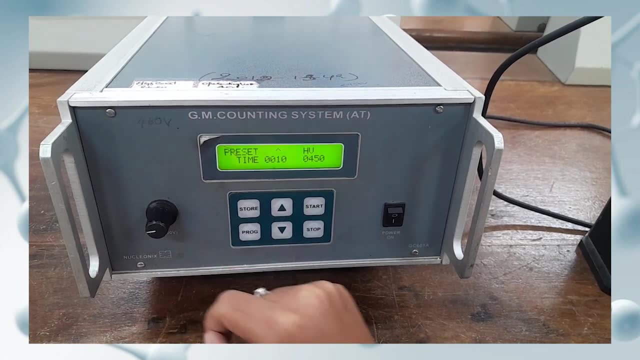 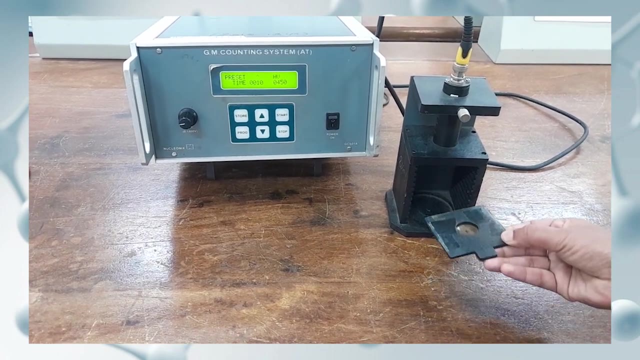 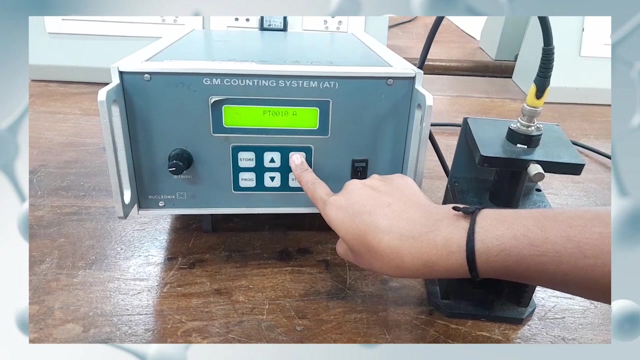 So now you have set the time, 10 seconds, and the voltage, 450 volts. Now we have to take the background count for this experiment. Take the first reading without any source, and press the start button. Record the number of background counts for 10 seconds. 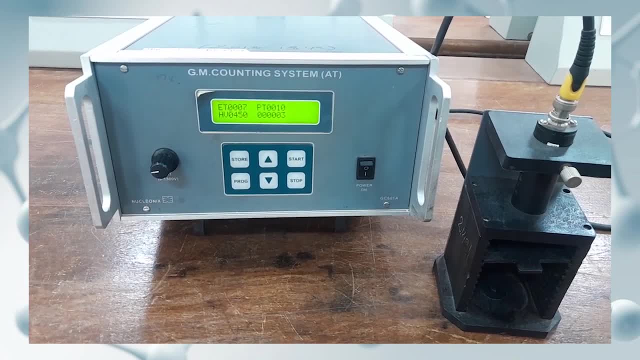 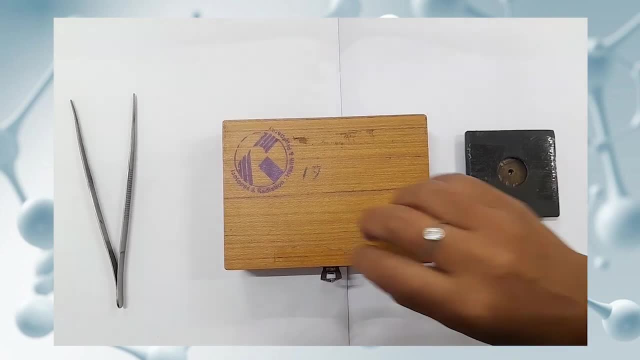 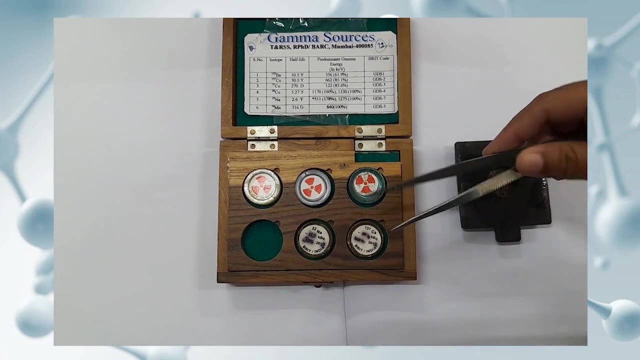 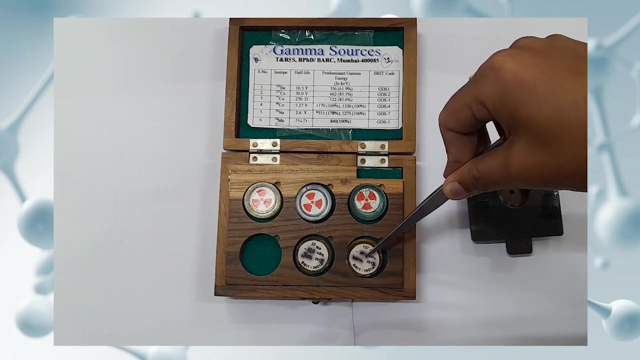 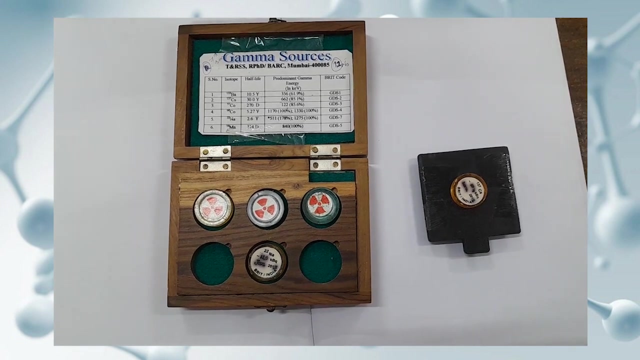 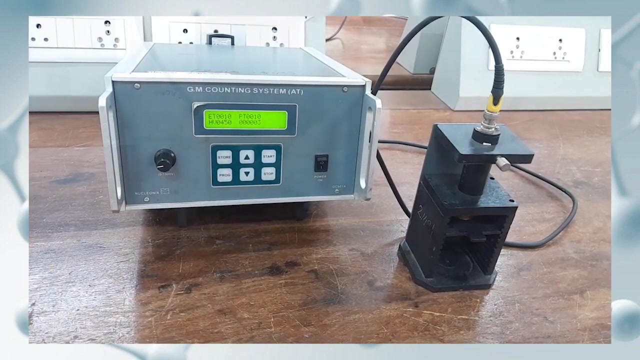 And repeat the same for 3 trials. Now let us place the source. The source used here is CCM source. Use a pair of forceps to place the source in the plate. Don't touch radioactive material with your bare hands. Insert the source at the fourth slot. 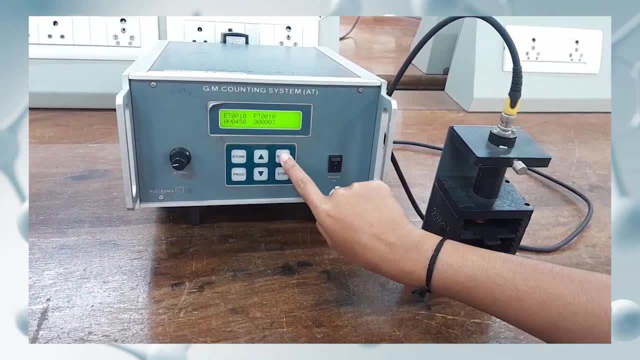 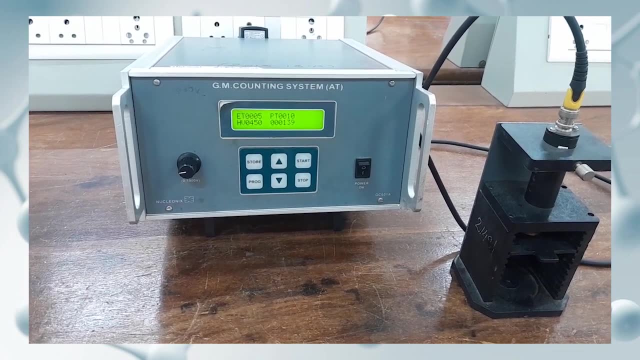 With the same settings of time- 10 seconds and voltage 450 volts. press start and take the readings. Repeat the same procedure for 100 trials. Now let us see the second reading. Now we have the same reading for the fourth trial, with the same settings of time- 10 seconds and voltage 450 volts. 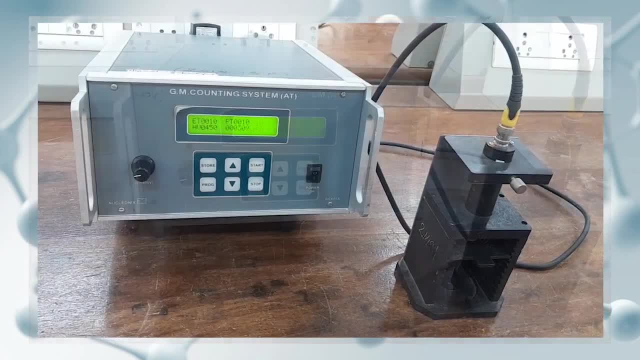 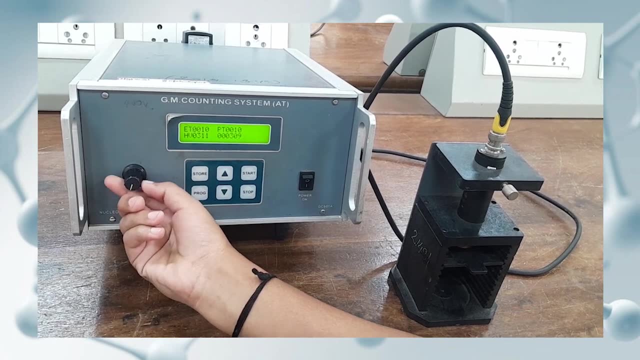 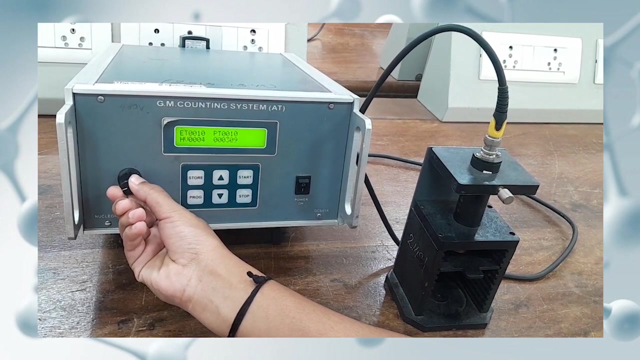 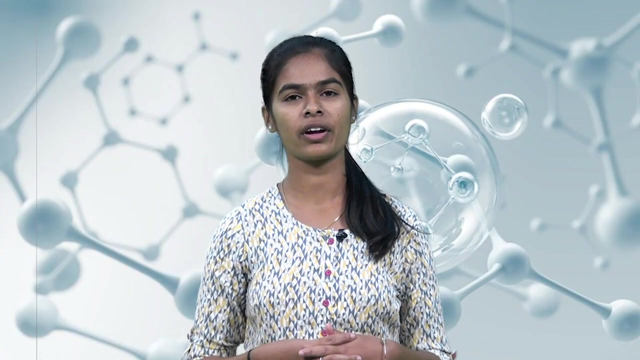 Press start and take the readings. Repeat the same procedure for 100 trials. Now you have to press the start button Now reduce the voltage to 0 volt by turning the knob on the gm counter and switch off the gm counter. We have recorded the trials. 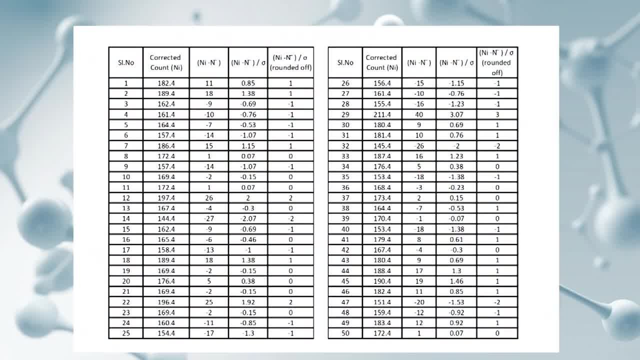 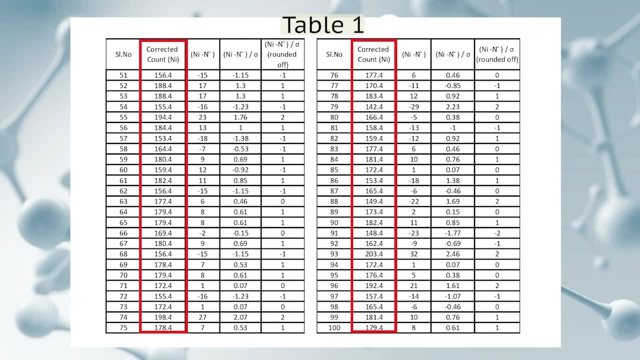 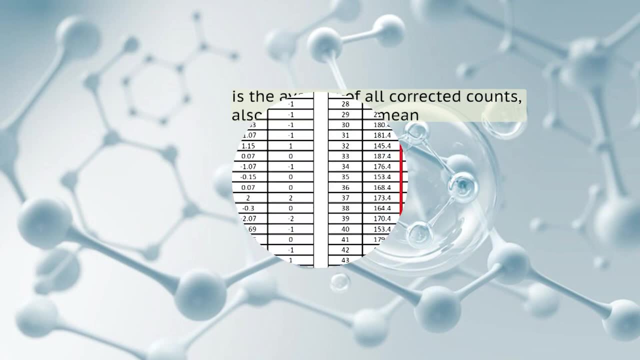 So let us see how to tabulate the readings In this first table. the first column is the observation recorded from the counter. Corrected counts. n. i is calculated by detecting the background counts from the measured counts. n bar is the average of all corrected counts, also known as the mean. 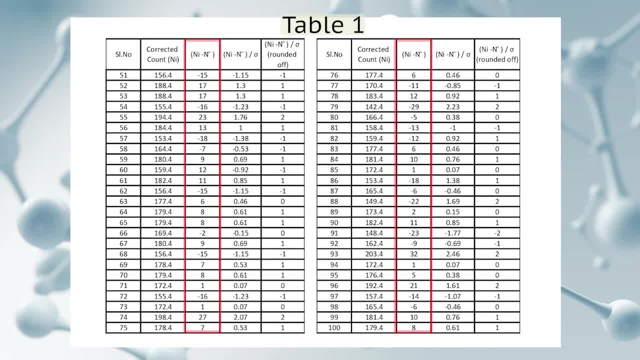 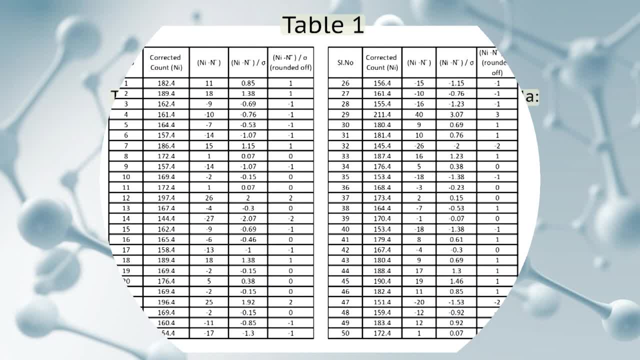 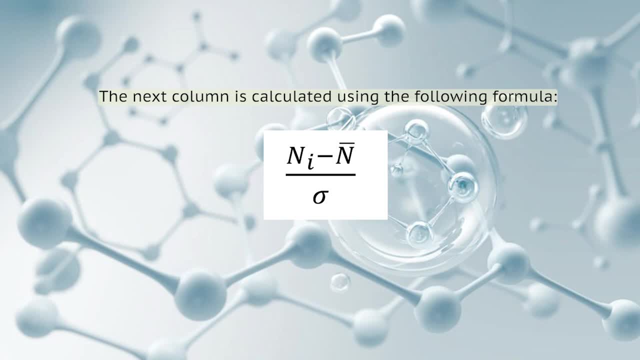 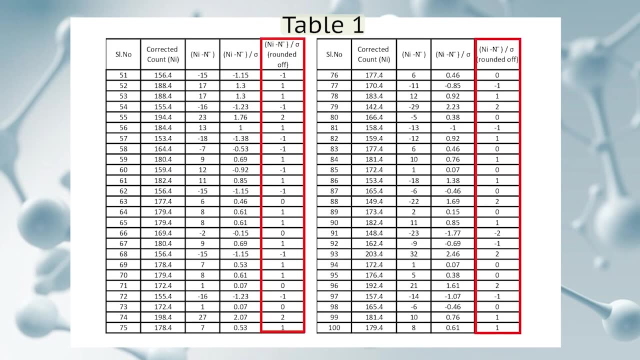 The next column is filled by calculating n? i minus n bar. The standard deviation sigma is calculated by square root of n bar. The next column is calculated using the following formula, that is, n? i minus n bar divided by sigma. The calculated values are rounded off to the nearest whole number and this is filled to. 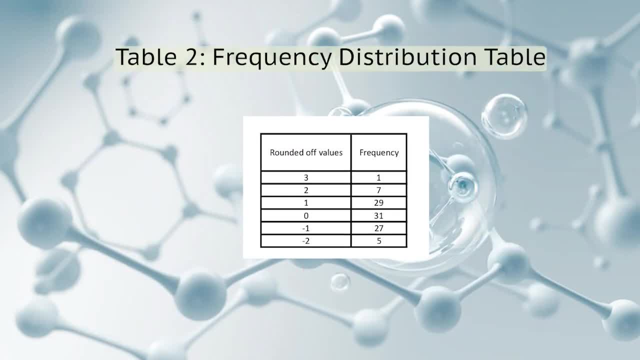 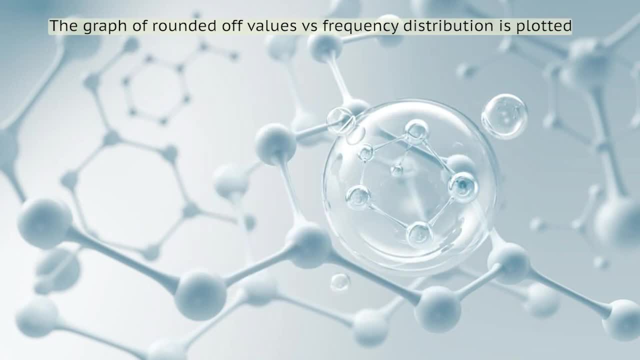 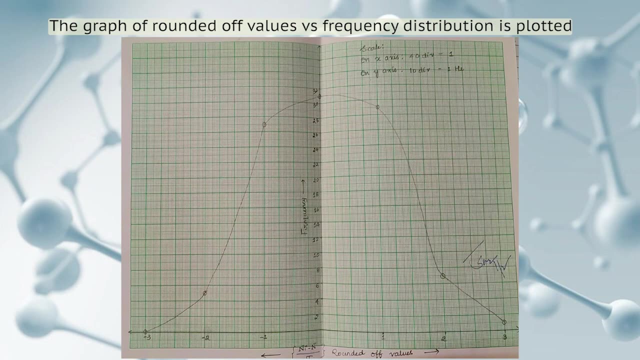 the last column. Using this data, we construct another frequency distribution table. The graph of rounded off values and frequency distribution is plotted and that comes out to be like this: Observe the graph displayed on the screen. The curve has a bell shape. 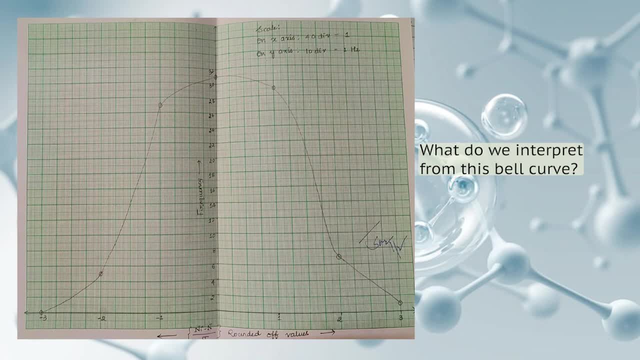 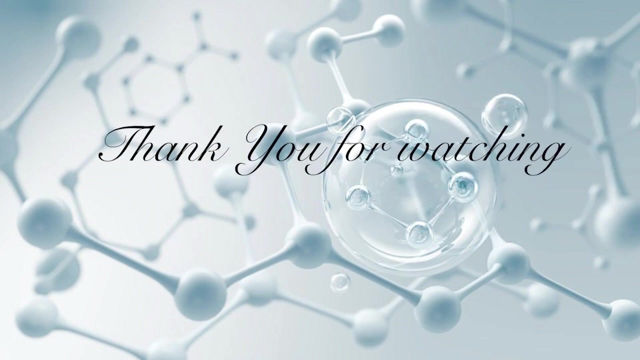 Now, what do we interpret from this bell curve? This graph shows that when the counts are high, we get a Gaussian curve, which denotes a normal distribution. Hence, this is the result of our experiment. With this, we have come to the end of our video. 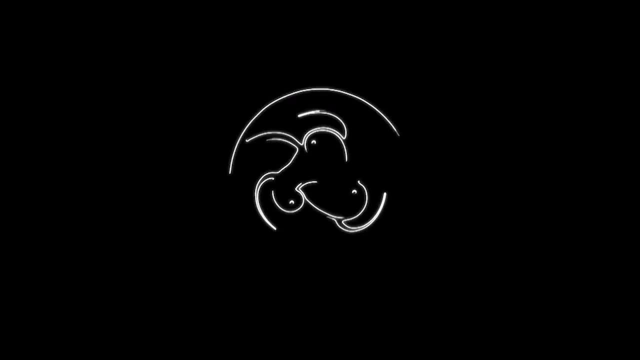 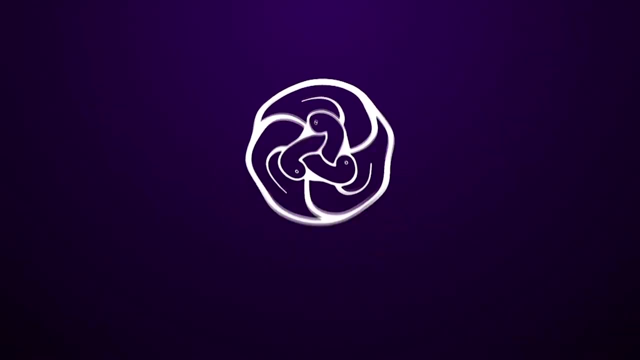 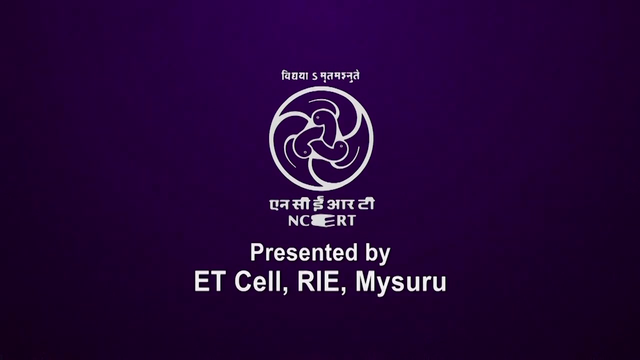 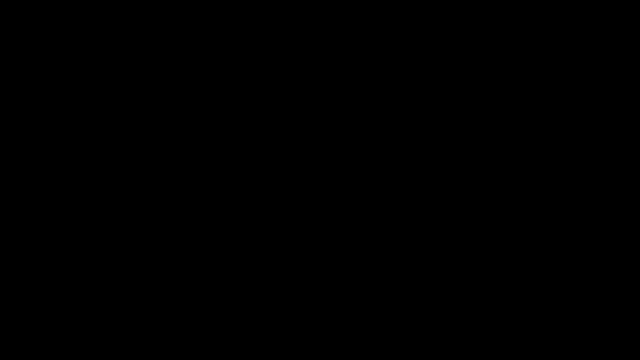 Thank you for watching. See you in the next video. Subtitles by the Amaraorg community.